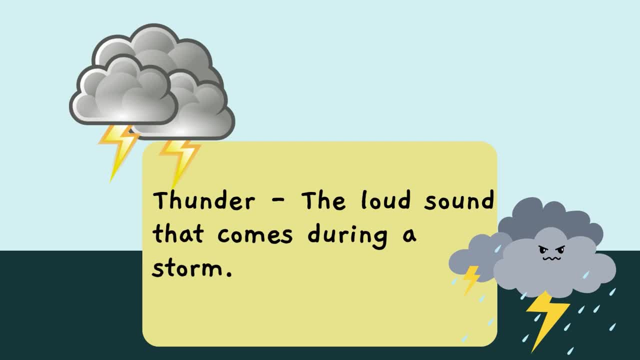 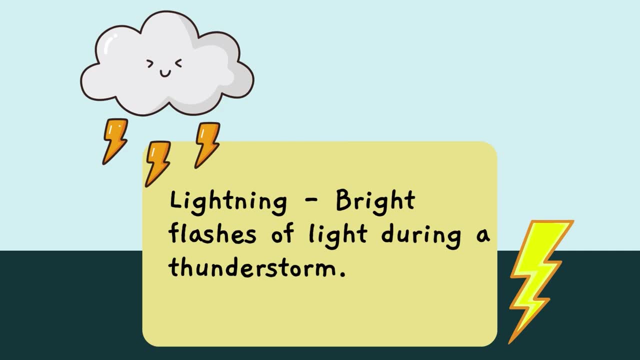 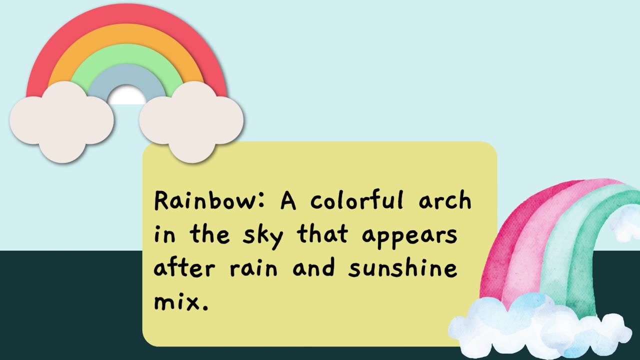 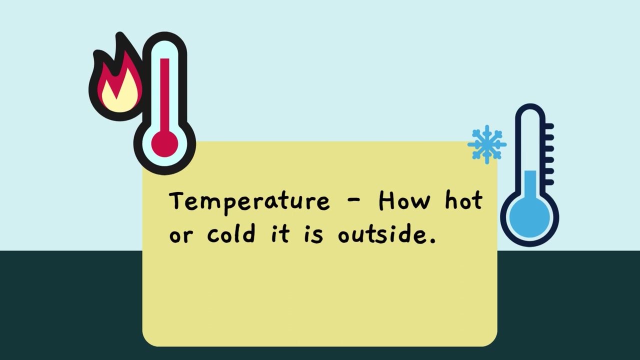 Thunder: The loud sound that comes during a storm. Lightning: Lightning bright flashes of light during a thunderstorm. Rainbow: A colorful arch in the sky after rain and sunshine. Temperature: How hot or cold it is outside. Thermometer: A tool to measure the temperature. 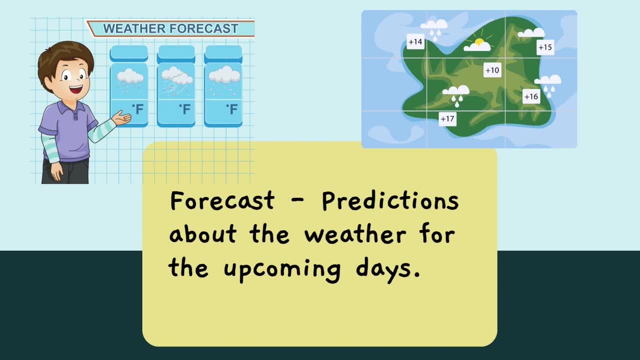 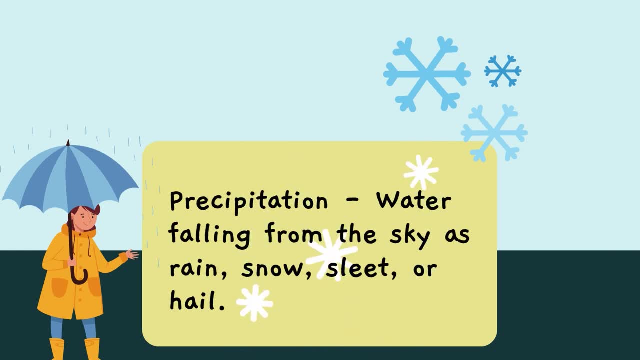 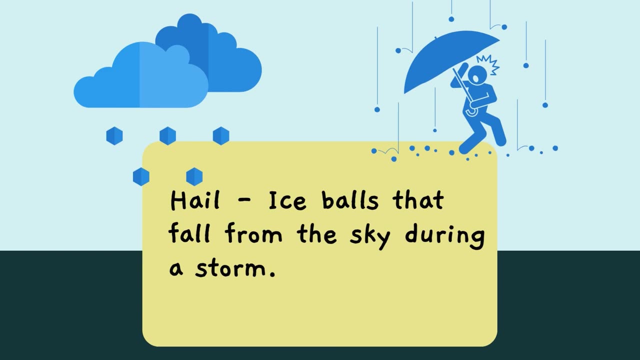 Forecast. Forecast Predictions about the weather. Weather for the upcoming days: Precipitation Water falling from the sky as rain, snow sleet or hail Hail. Ice balls that fall from the sky during a storm Blizzard, A strong snowstorm with lots of snow and strong winds. 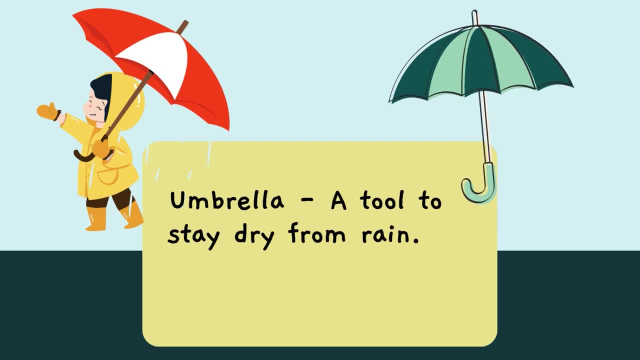 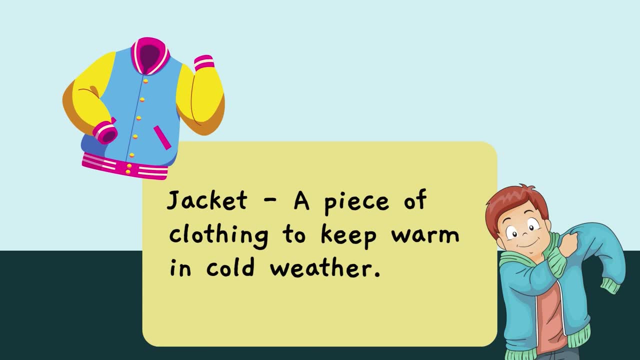 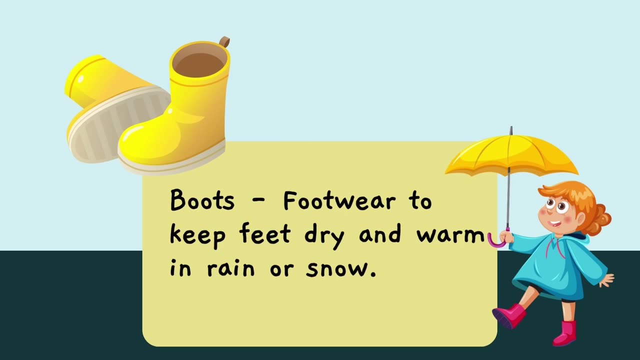 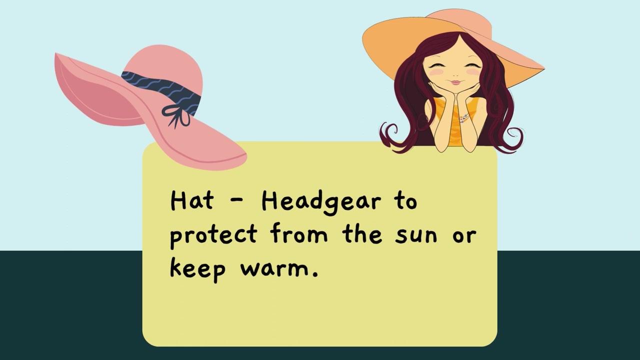 Umbrella, A tool to stay dry from rain. Jacket, A piece of clothing to keep warm in cold weather. Boots, Footwear to keep feet dry and warm in rain or snow. Hat, Headgear to protect from the sun or keep warm. Gloomy, A dark and sad-looking sky. 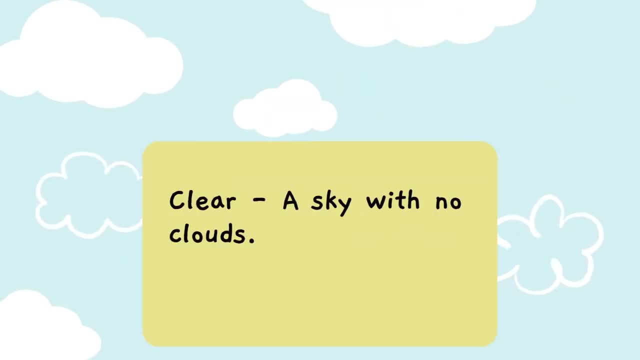 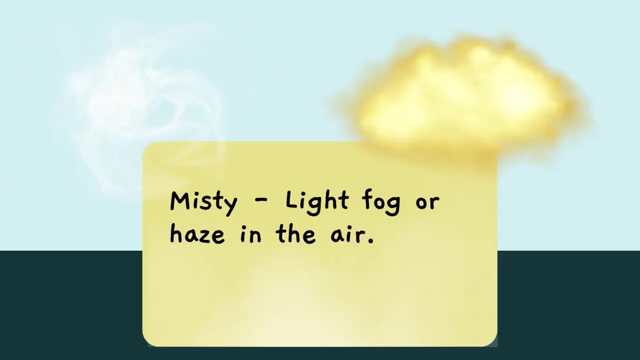 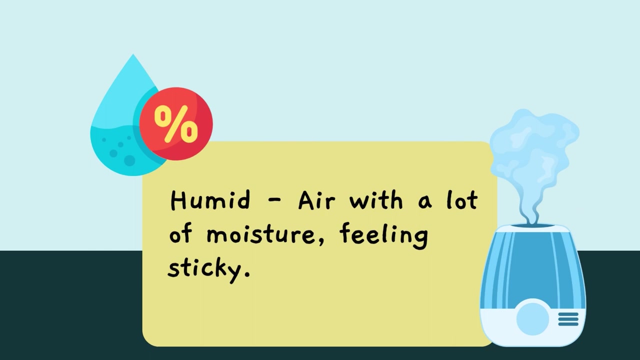 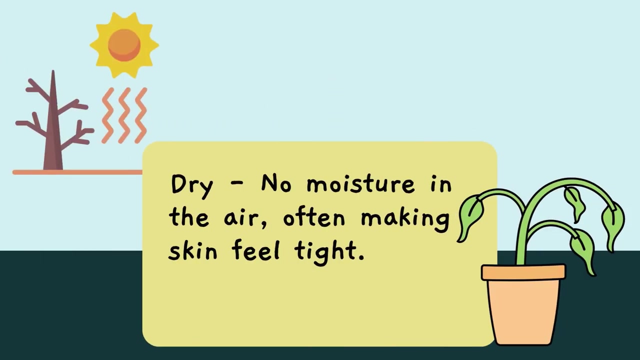 Clear A sky with no clouds- Clouds. Here are the five signs for a Parte 1 weather forecast: • Misty, light, fog or haze in the air. • Humid air with a lot of moisture feeling sticky. • Dry, no moisture in the air, often making. 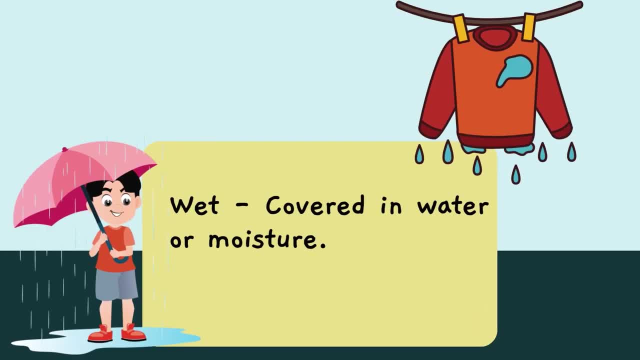 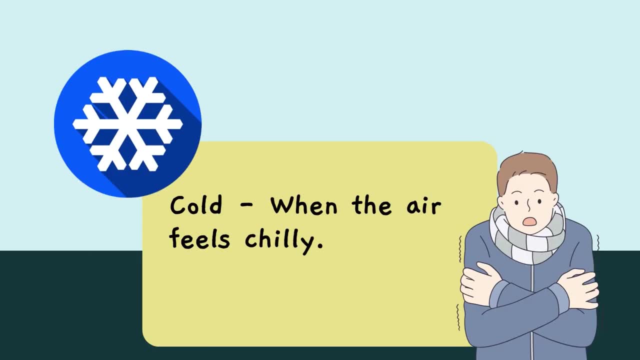 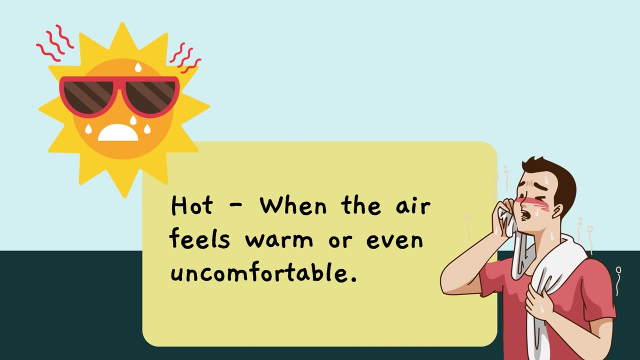 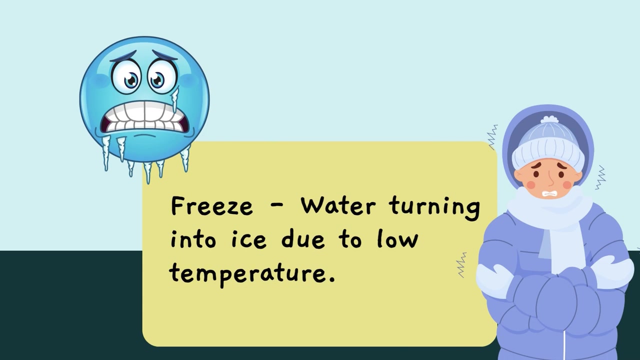 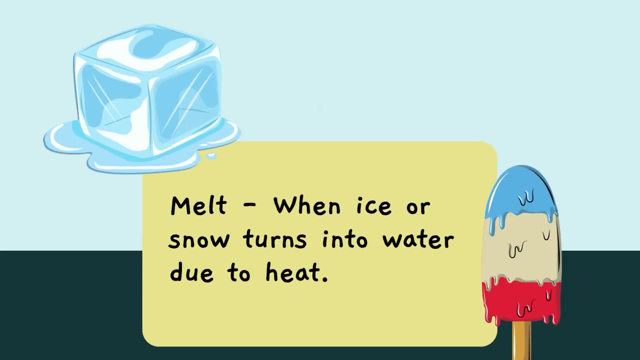 skin feel tight. • Wet, covered in water or moisture. • Cold when the air feels chilly. • Hot when the air feels warm or even uncomfortable. • Freeze water, turning into ice due to low temperature. • Melt when ice or snow turns into water.